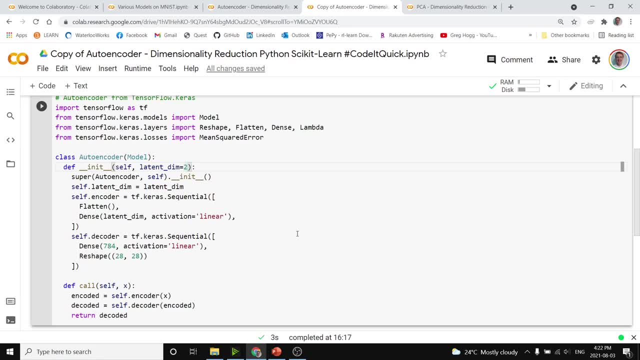 parts of this, So let's go ahead and do that. So we're going to paste a bunch of code here and I'm going to explain all the important parts of this, So let's go ahead and do that. So I pasted this because it's not too important. of all the specifics here, I'm just going to point. 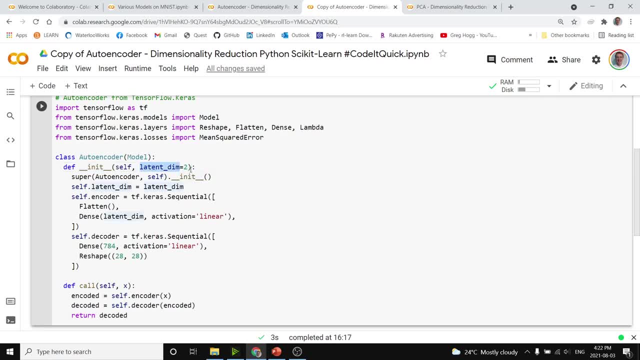 out the particular pieces. In the init function we have a latent dimension which we set equal to 2. That's the same thing as end here, and it's very important to know the number of dimensions you're going to convert it into. And then we have the encoder and the decoder, And so in the encoder, 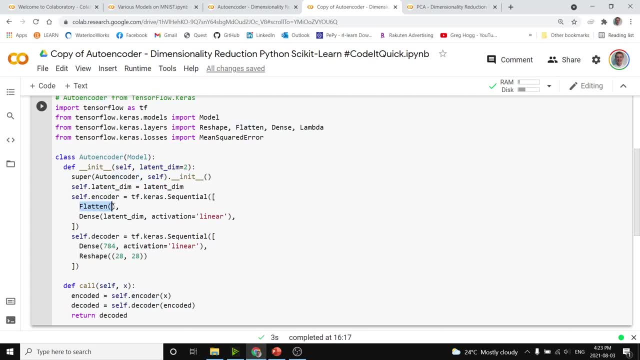 step. that is going to be the beginning of the network, and so we're going to just flatten it and then call dense with linear activation of convert that into the number specified by the lat and dim. That is what we're going to call. We'll call selfencoder or autoencoderencoder. 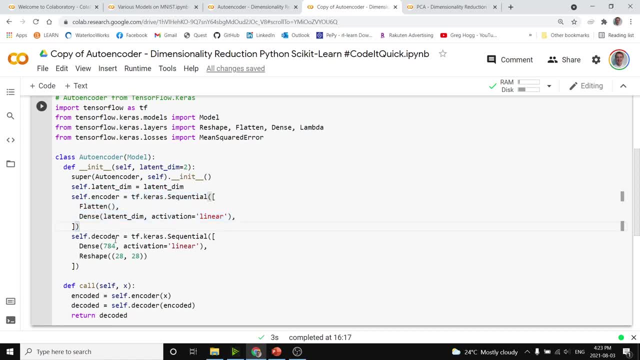 when we want to actually do the dimensionality reduction, We also need the selfdecoder for training the model, and so that is going to come after the encoder step, and it's going to be whatever the dimension was to begin with. And so that is the flattened version of 28 by 28,, which 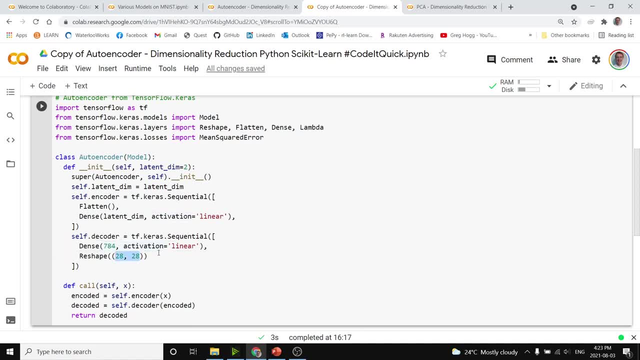 is 784, and then we reshape it properly back into 2828. And so we specify down below with call, and what that does is: it makes it a little bit easier for us to do that. So we're going to make the encoded and then the decoded and then it returns decoded. So to use this model, 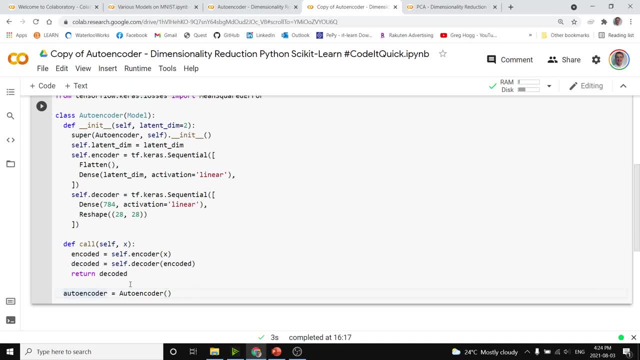 we will first make an actual instantiation of it, and so we'll make autoencoder equal to calling autoencoder, And then after that we do autoencodercompile with: set the optimizer equal to probably atom and the loss definitely equal to mean squared error. And now we need to. 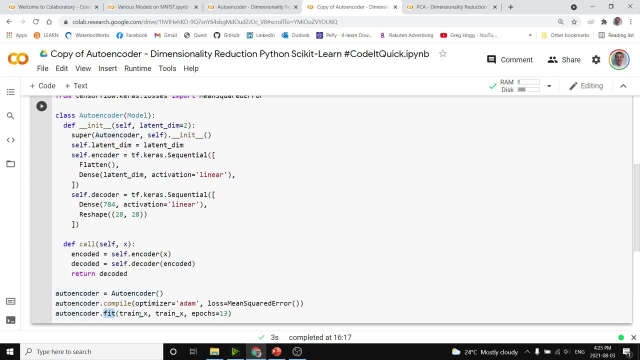 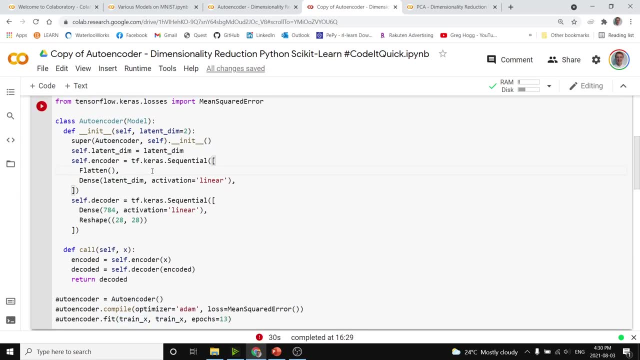 fit the model, and to do that we simply call autoencoderfit, and then we pass the input and the output as the exact same thing, which is both the input And, although it might not be totally necessary, generally what we do after flatten is we apply a lambda function. 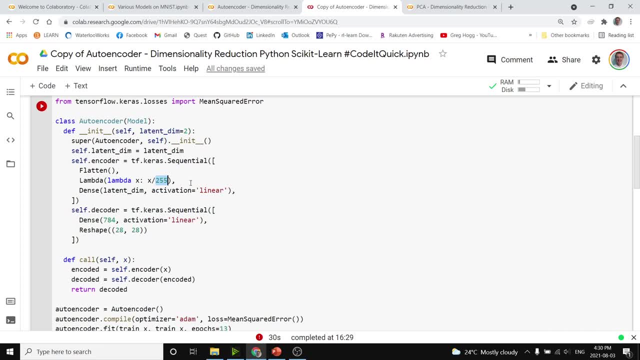 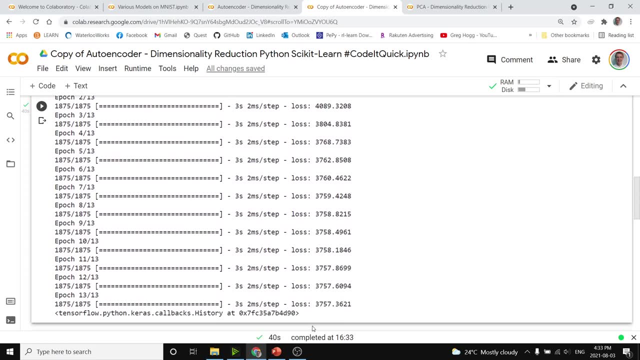 where we divide each of these by 255, or whatever. pre-processing normally makes sense for your problem When fitting the model. if you don't see the loss go down and kind of balance out at some point, then you probably did something wrong. Now the main point of our encoder is to actually get 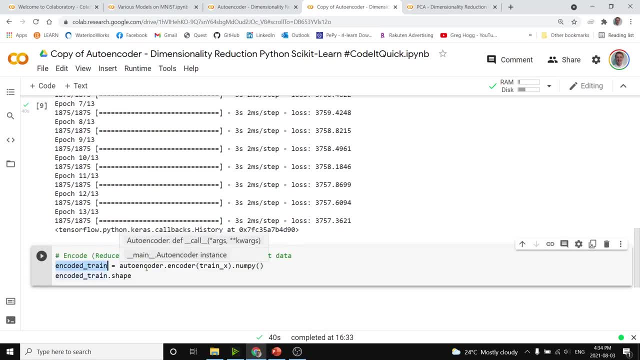 encoded data and we do that by doing. encoded train is equal to autoencoderencoder, so then it calls the encoder piece, we pass that to our training examples and then we do that to numpy, So after that we can use autoencoderencoder. and then we pass that to our training examples and then we do that to numpy, So after that we can.